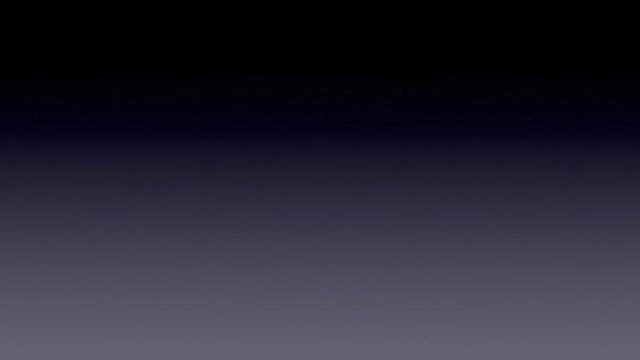 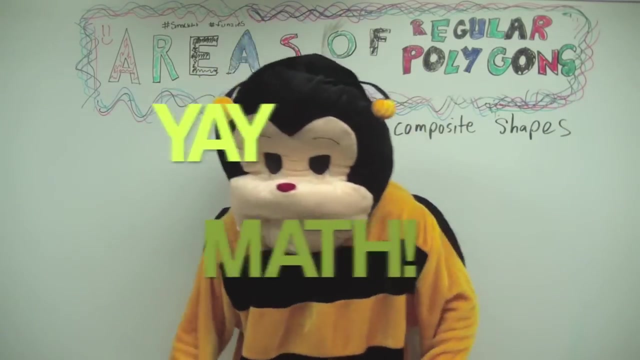 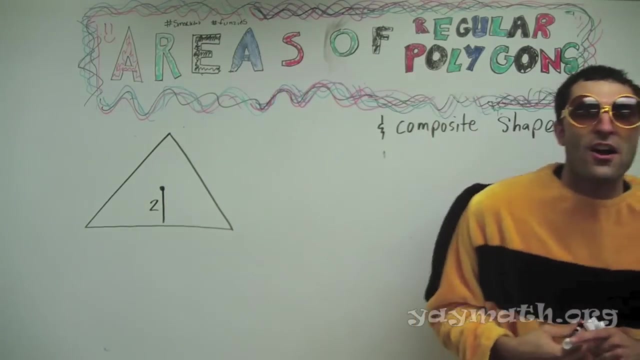 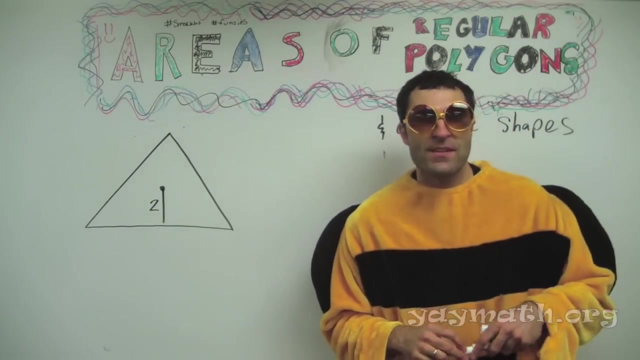 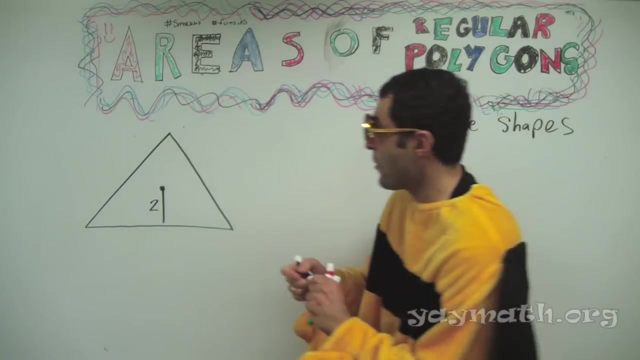 Please draw the last shape. we're going to do: Equilateral triangle. Is it okay if I go in the back? Yeah, please Use as much space as you need. Equilateral triangle. Notice that the sides are not given. I'm going to say that it is equilateral so we can mark that. 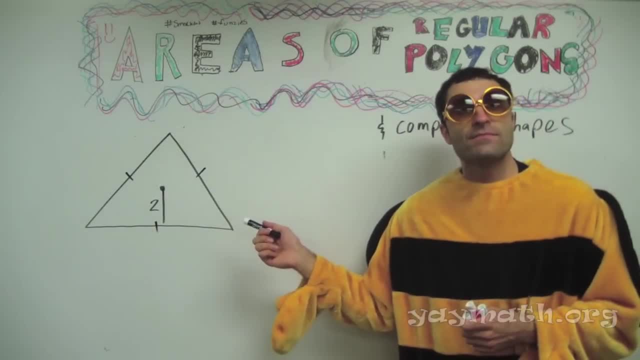 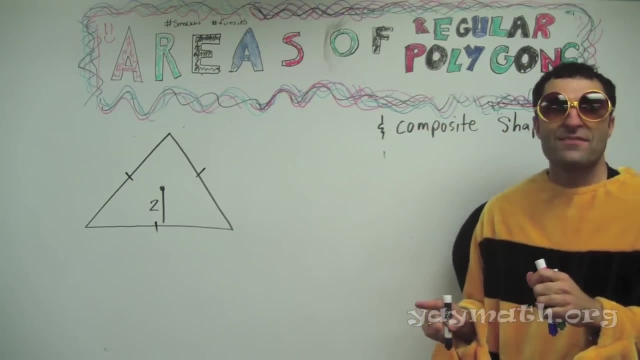 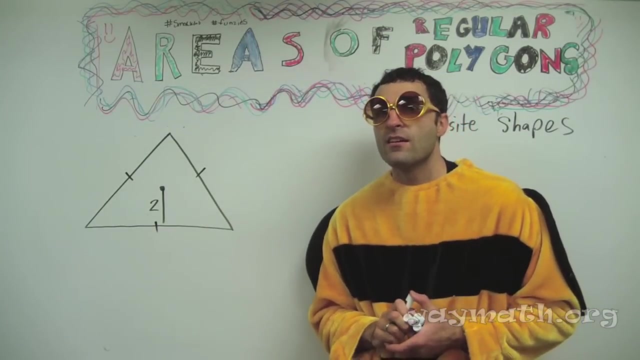 The sides aren't given, but what is given? Radius, That would be if it's a circle, No, it's a midway pointer, Half of the altitude, Apothecary, What's the thing that's like? the length, Altitude, No, Height. 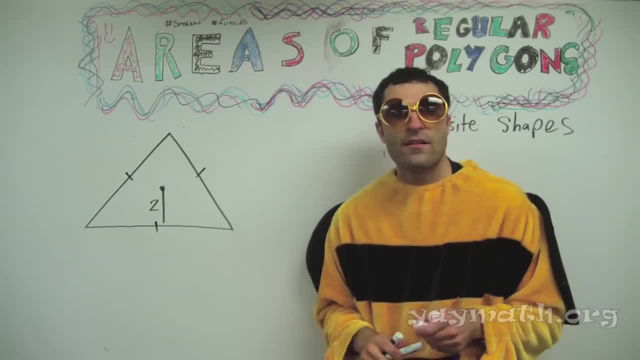 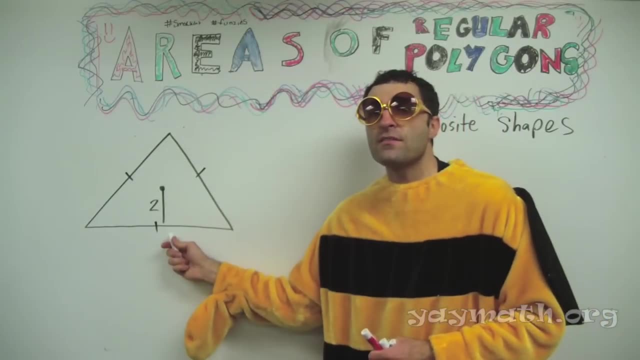 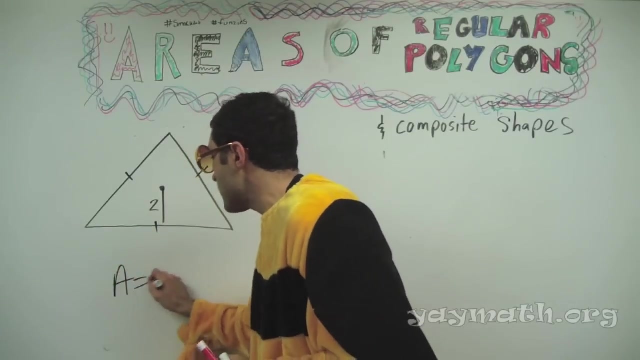 Median. What are you asking for? Are we going to the bisector? Okay, we'll come back to you. Apothem is given. So we want the shape, the area of this triangle. Normally, you guys, the area of this triangle is 1 half base times height. 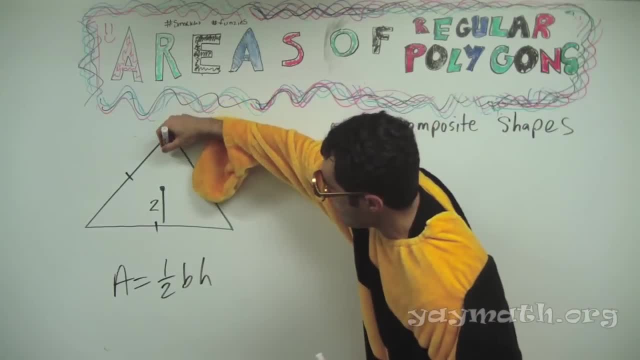 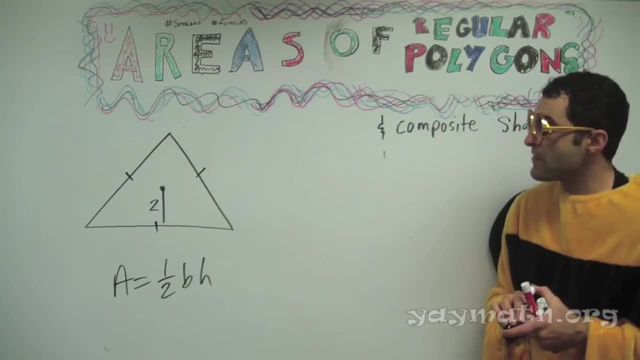 If you're able to get this whole height, that's great. There are ways to do that. Can we just double the apothecary? No, it's not Good guess. It's not. That's a really good guess though. 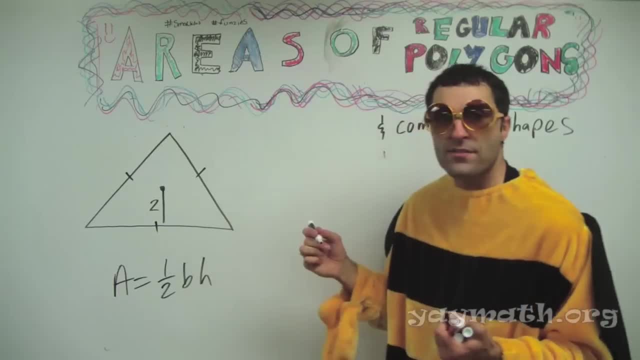 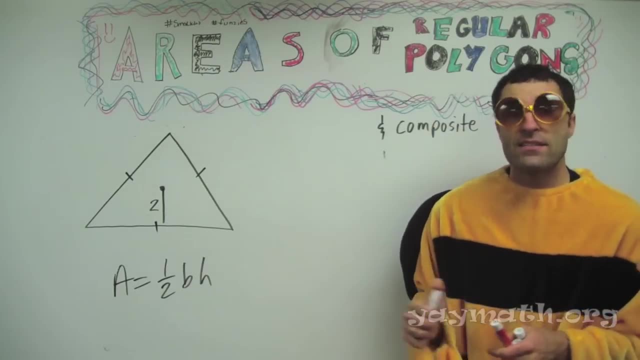 Let's find out what it is. Yes, So is that point in the middle a midpoint? or is that just a point, Assuming it's the height based on the middle? Yes, it is the middle, So then it shouldn't be doubled then. 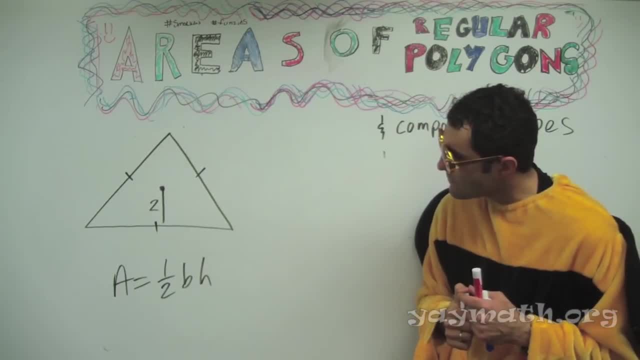 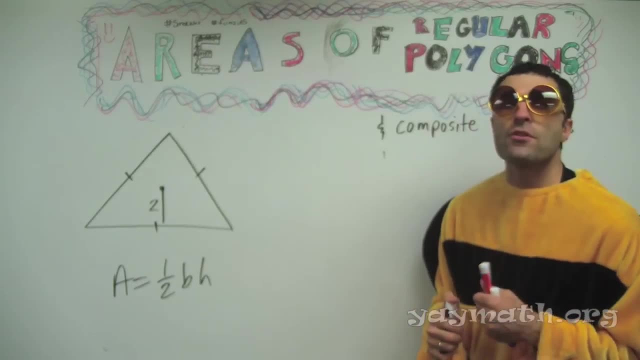 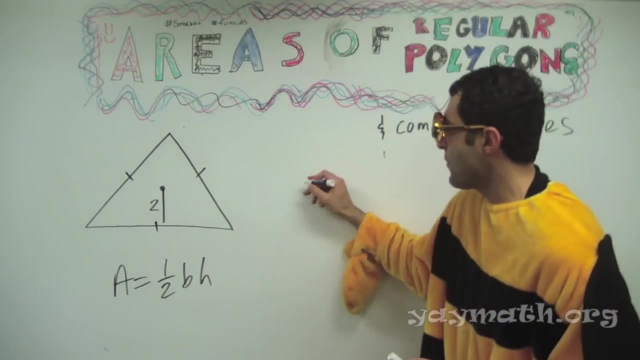 It would make the total height of the triangle, Because if it's a midpoint, shouldn't that be exactly half the triangle? You know what? Let's find out. Maybe both of you are right Now. instead of using this, let's try the 1 half. 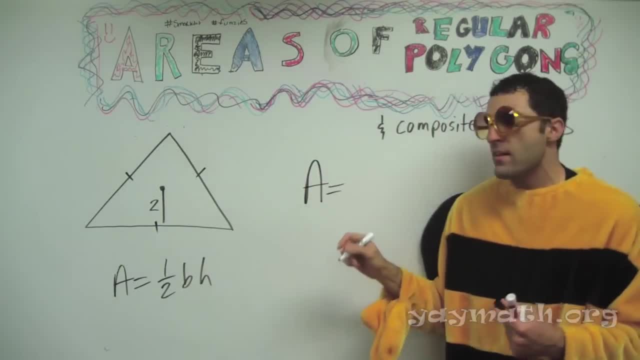 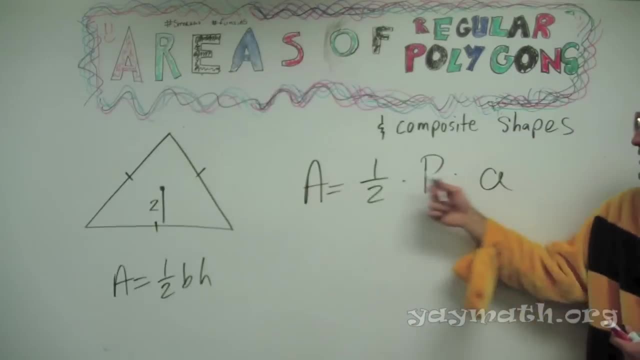 Notice. it's a positive practice. It's a good practice to put 1 half, Put the formula down and then work on what you need to get. Do we know anything already? We know the apothecary, so you can put 2 in. 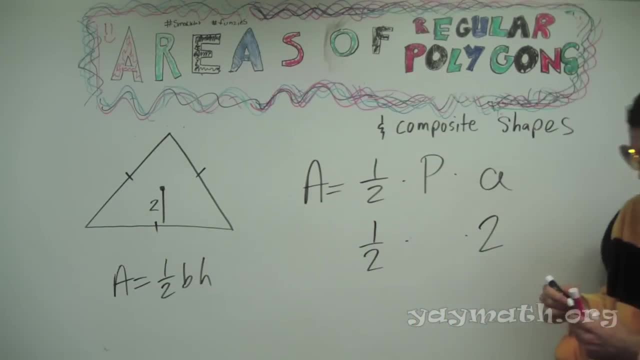 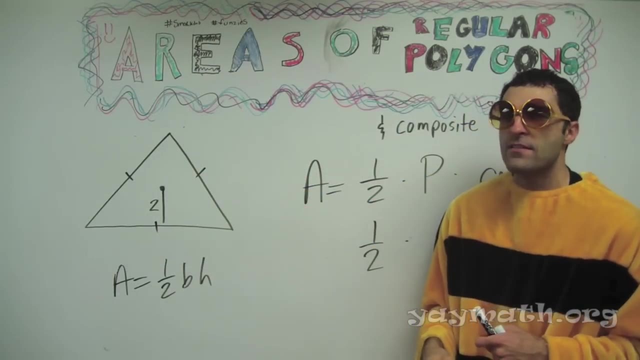 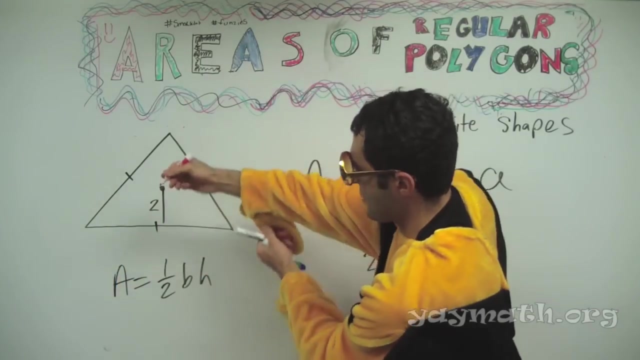 So 1 half times. So we need the perimeter. Okay, Now we could do the 360 divided by how many? in this case 180.. How many triangles would exist? There's 4 triangles in there, though 3, actually I'm going to draw these. 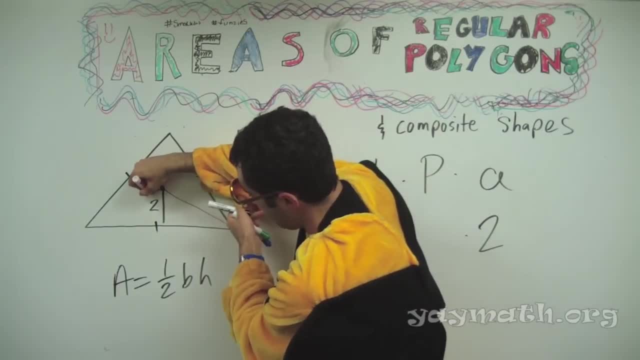 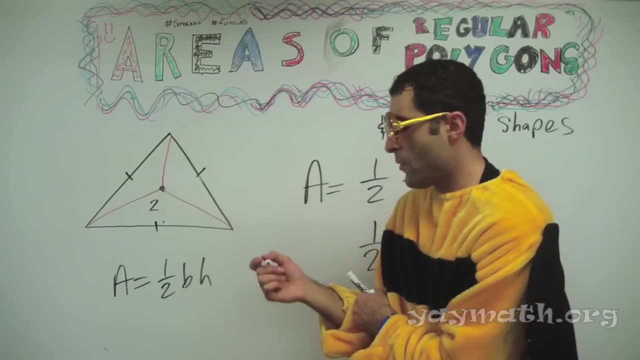 There's 4.. There's stress: The triangle is. within that There's 4 triangles, So I like 3.. That's what the idea of 3 is. But what you can do is How many sides there are, that's how many triangles there can be. 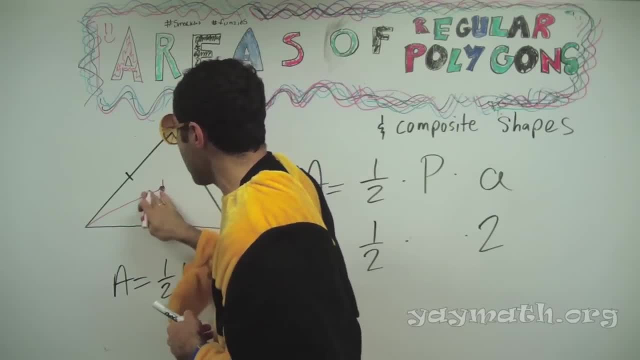 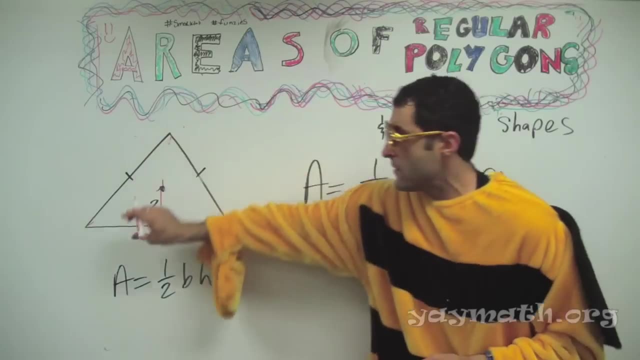 Yeah, that's right. That's basically the idea. You divide by the number of sides. However, there's a quicker way: Equilateral triangle. Equilateral triangle: Each angle must be what The same, Making it 60.. 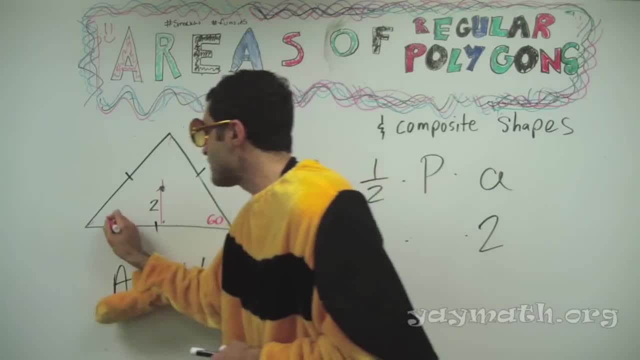 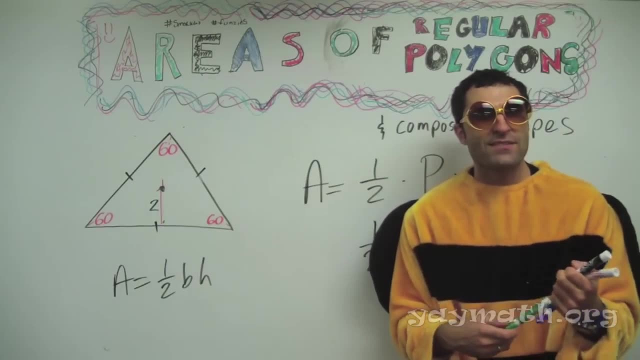 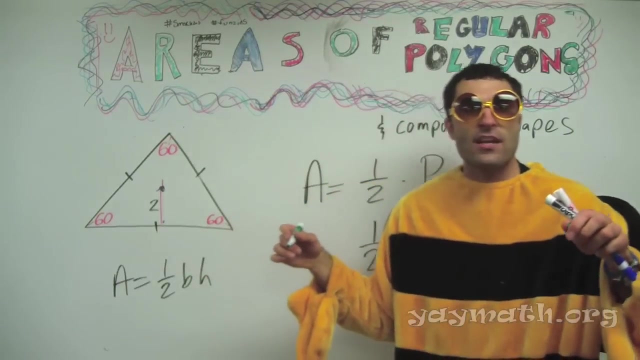 60.. Putting it down, Each of these are 60.. Thank you for the sound effects. I'm sorry I dropped my pencil, So that's 60.. How do we get sides, Suggestions, Suggestions, Oh no, I don't know. 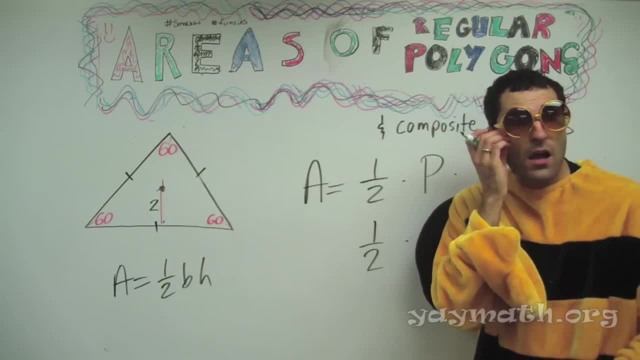 Go back, Go ahead. I'll come back to you. Go ahead. 30, 60, 90.. It is a 30, 60, 90. Where do I draw it? The 3 triangles that you can make: 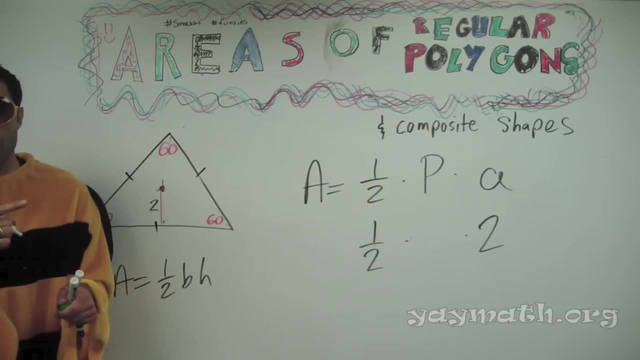 Well, the 30,, 60,, 90 degree will be a 90 degree triangle in there, A right triangle. Good, This is your 90 right there. Oh yeah, Where would the rest be? Up All the way up. 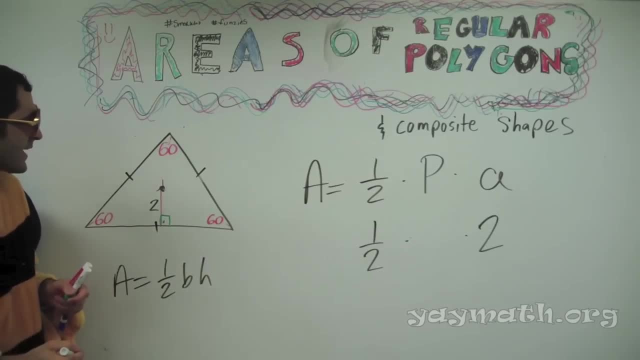 Yeah, That could work. Yeah, That could work. but we don't know this whole side. Can I show it to you? Yeah, What are you going to say? I was going to say you draw it from the midpoint to the. 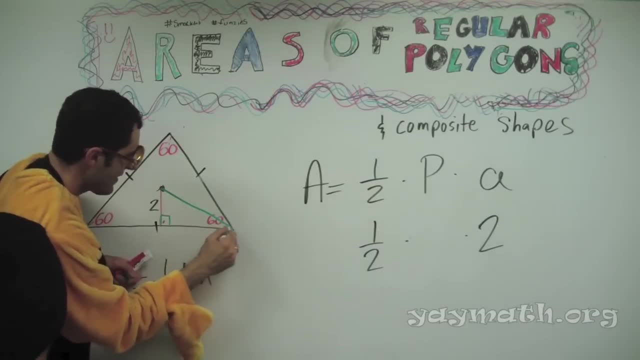 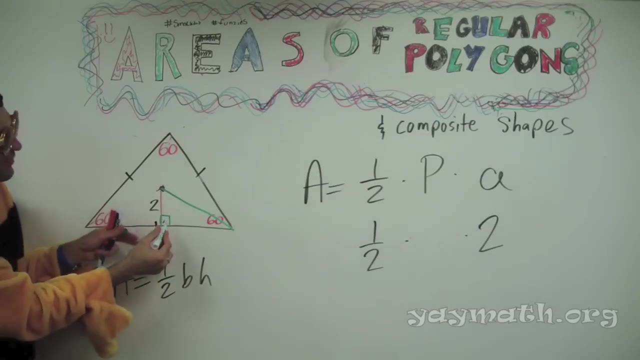 Yeah, from the midpoint over. Check that out All right, Because we have this side. If we drew all the way up, we don't have one side. Does that make sense? Yeah, Okay, So here's 2.. What angle is this? 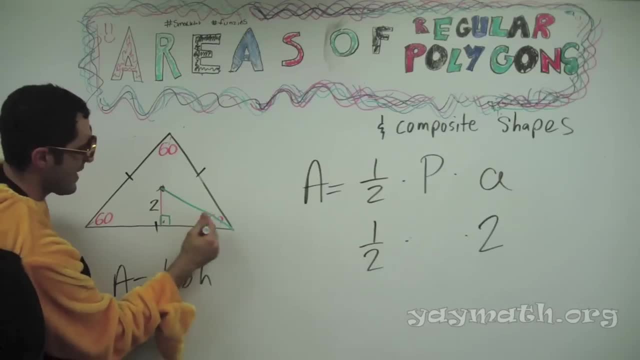 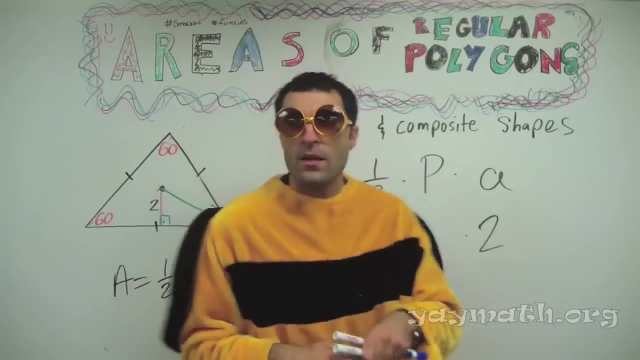 30.. 30.. Putting it down: 70.. Just a smidgen. Okay, Now you can fill it in. Great, This is 30.. 2 is the 30th triangle. 2 is the 30 side. 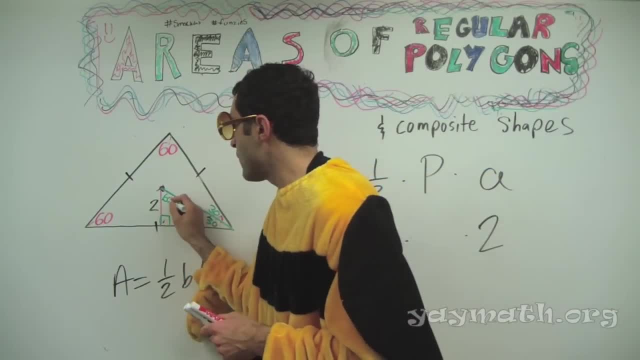 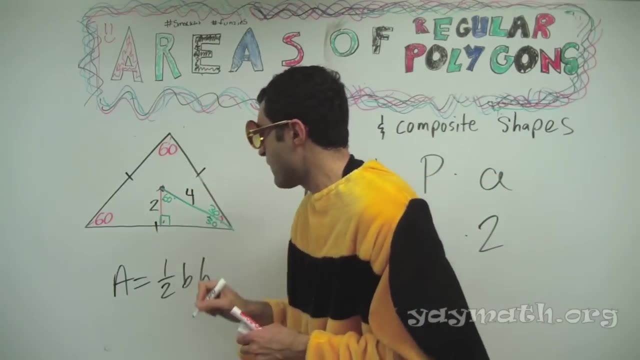 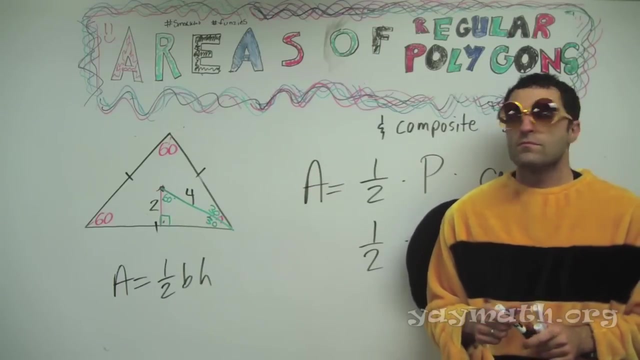 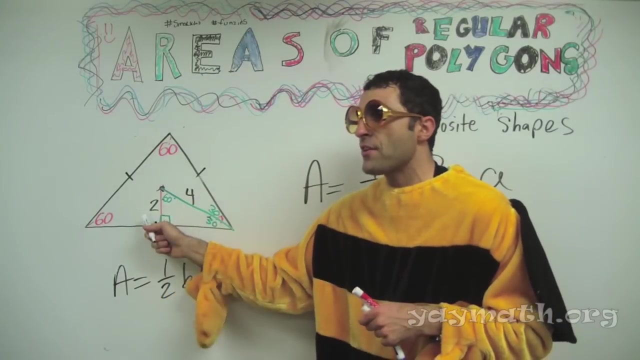 So I know the hypotenuse is going to be 4, and I then know that the 60 side will be 2 root 3.. Good job, Scotty. Yep, Yes, Let's talk about it. If you're at the 30 degree side, that's 2, the side opposite 30. 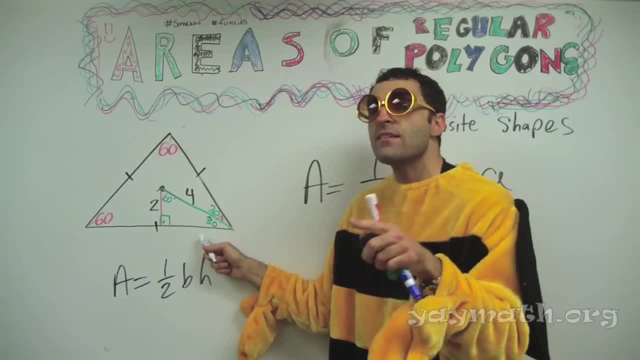 To get the side opposite, 60,. you multiply by 2.. Multiply by Root: 3. Root, 3. Root, 3.. So that's 2 root 3. is this particular side? Indeed, 2 root 3 is that particular side. 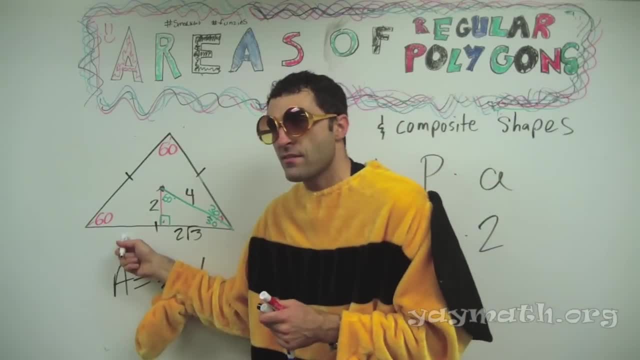 Indeed. So if that's 2 root 3, what's this? 2 root 3.. What's the entire side? 4. Say it: 4 root 3.. 4 root 3 is the entire side, Which means that every single side is 4 root 3.. 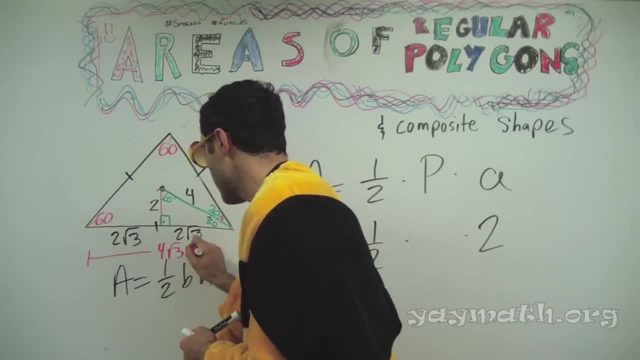 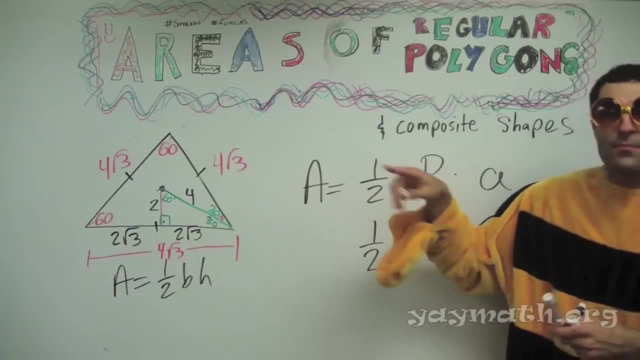 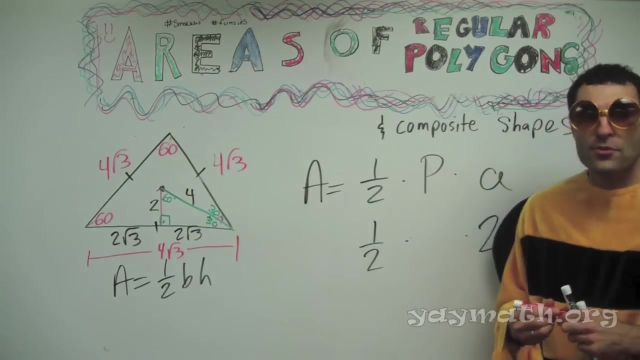 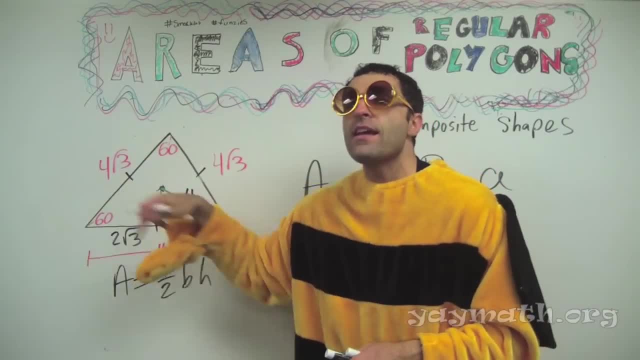 1 root 3.. Oh, Oh, Oh, 1 root 3 plus 4 root. 3 plus 4 root 3 is not the middle. Ohh, 12 root 3.. Root 12 root 9.. 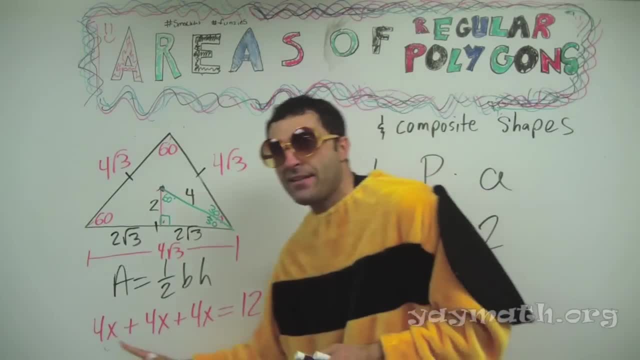 3. 3, 3. You add it: 4 root three plus 4 root 3 plus 4 root 3 is 12 root 3s. just like this is true: 4x plus 4x plus 4x equals 12x. 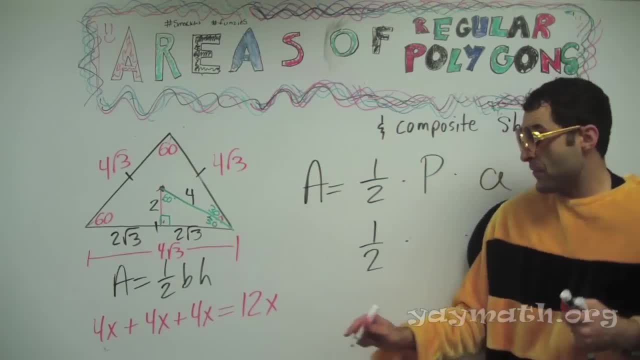 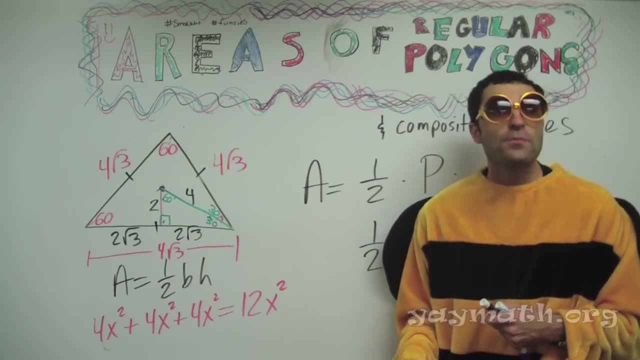 Now notice: I didn't change x when I add. I group them. Because you have 12 x's, We have 12 root 3s. Also like x squared, Very nice. Same with x squared, Bravo. Multiplying is a different story, correct? It's not a grouping anymore if you're multiplying. 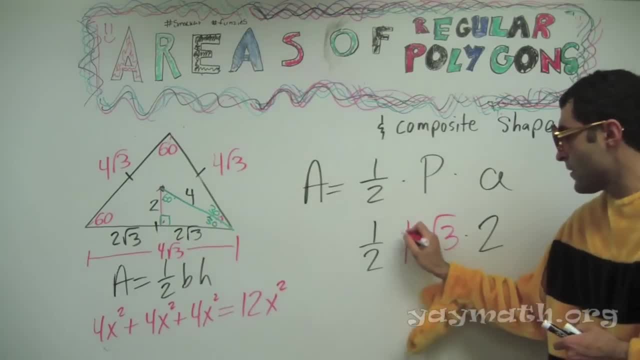 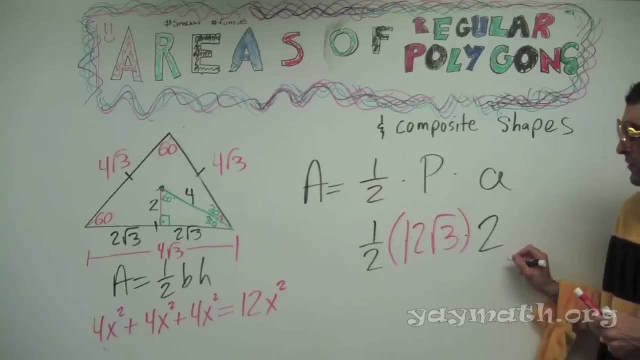 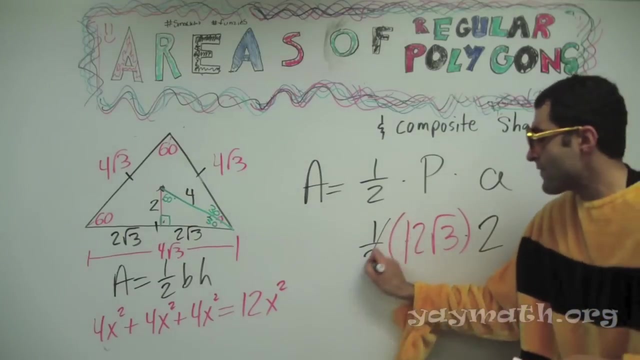 So we're putting 12 root 3 here. bravo, Okay. Finally, what do we have? 6 root 3 times 2 makes 12 root 3.. I also like the half times 2, they go away, leaving 12 root 3 alone. 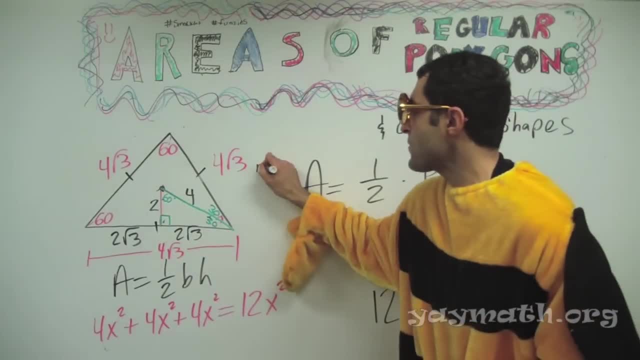 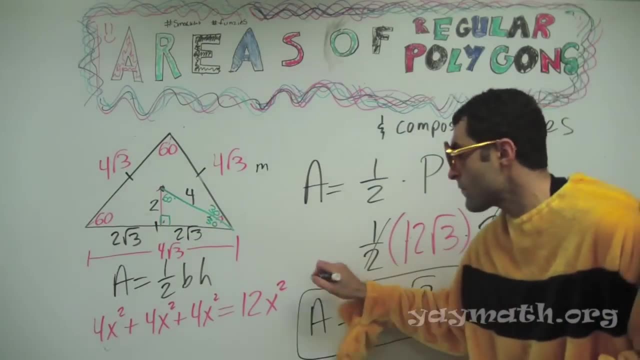 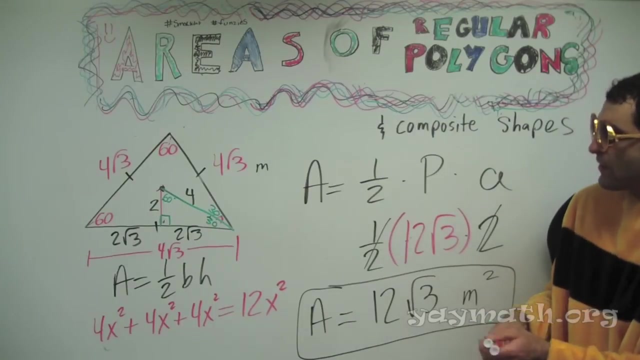 12 root 3,. let's put it down in meters. meters squared is the area. Okay, Now let's figure out whether or not this is double. shall we? That was your question, We shall. So if this is 4, do you agree that this triangle you create here? 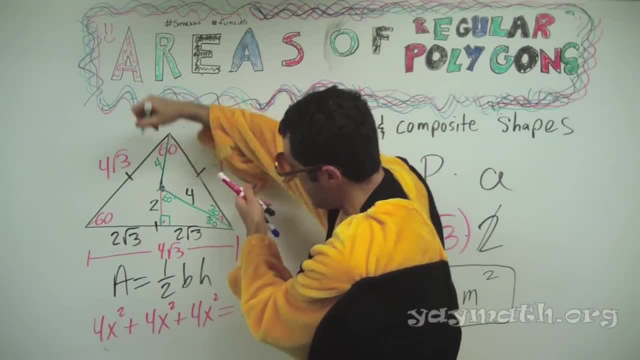 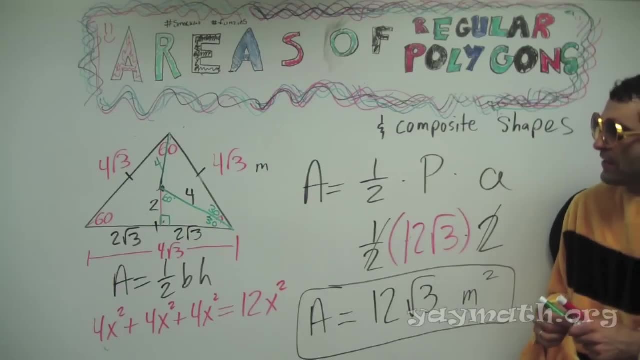 that this would be 4 as well. It's the size of the triangle. Yeah, so the entire height is 6.. The entire height is 6. Which would still work, because if you did 1 half base times height, you're still going to get the same answer. let's find out. 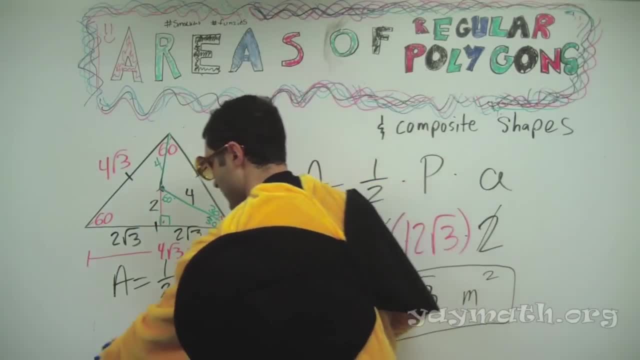 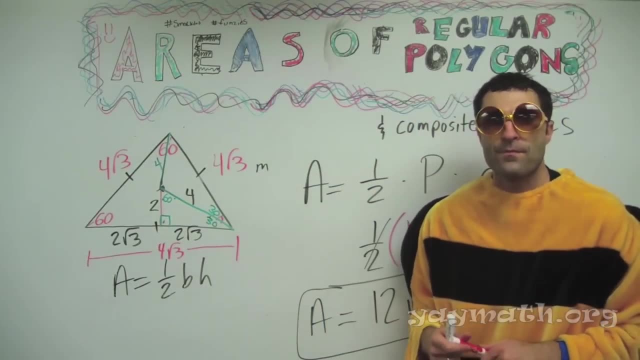 So wouldn't it be safe to say that you basically double the apothem and then basically add the apothem and it's doubled together. I think that's a safe assumption for an equilateral triangle. yes, So only for equilateral triangles. 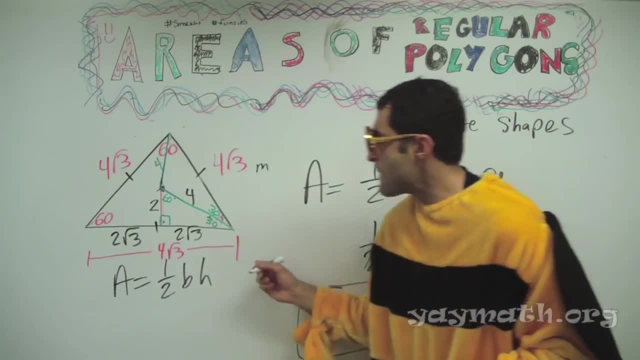 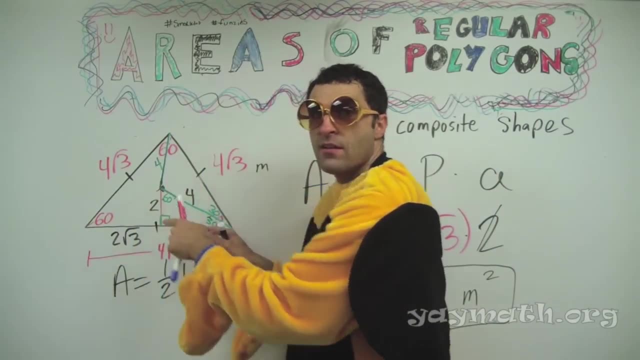 Yes. So then, technically, isn't that not a correct midpoint? Because if it's a real midpoint, wouldn't it be just doubled, in that It's midpoint to each of the vertices Period, Like you spin it on a wheel, If you were to spin it on that dot, the dot would move. 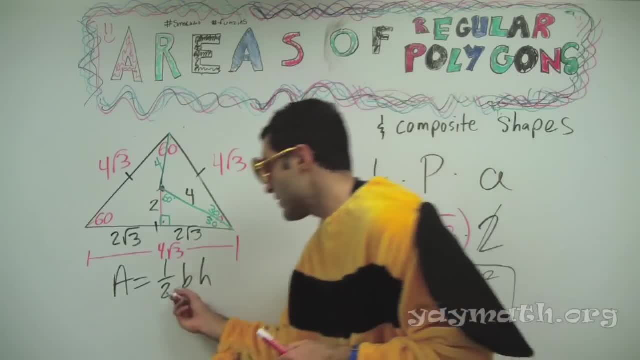 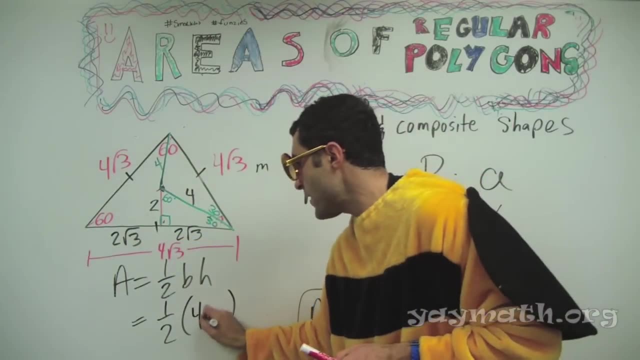 That's like a perpendicular vertical right. Yes, Yes, Let's put it down: 1 half. the base would be what 4 root 3.. 4 root 3. And the height Is 6. 6.. 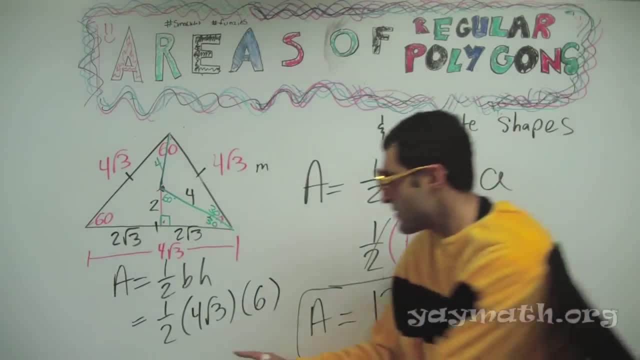 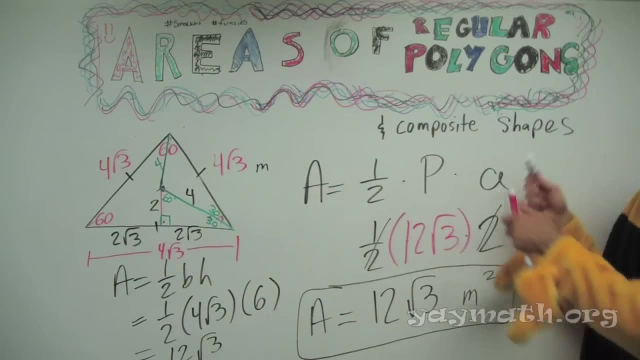 Does this work? It does, It does. So this is 2 root 3 right here, multiplying times 6, 12 root 3.. All right, There's one little caveat that we're going to add, and we're almost done. 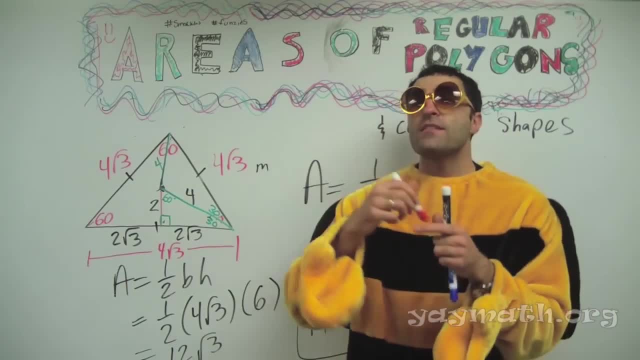 Composite shapes. Here we are. What if I want you to draw, please? Is B-man coming back? Can we do one of like these? We're doing it right now. Oh OK, Good job, Let's call it a composite shape. 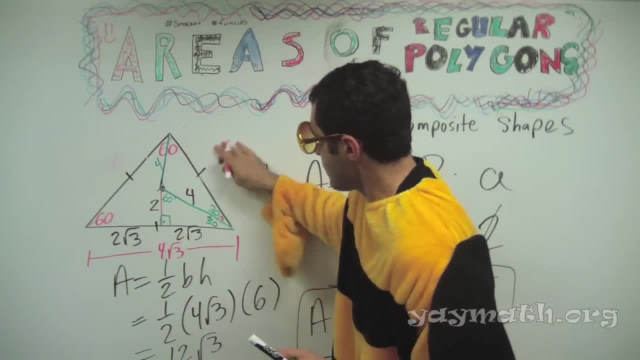 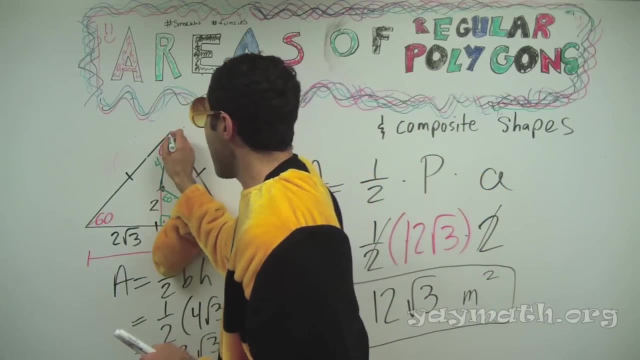 Thank you for asking. Is B-man coming back? Composite shape: Here we go. What I want you to drew drew. what I want you to draw is a circle around this. Oh OK, Oh Lord, Oh Lord. 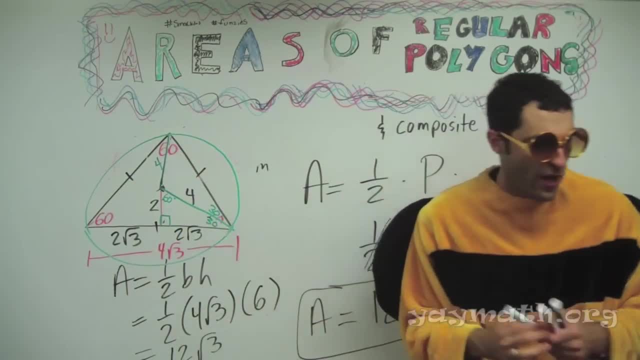 Oh Lord, Circle around the triangle. Oh Lord, Circle around the triangle. I'm going to erase a little to make it easy on the eye. Yeah, Then a little goes here So we have a little bit of space on this. 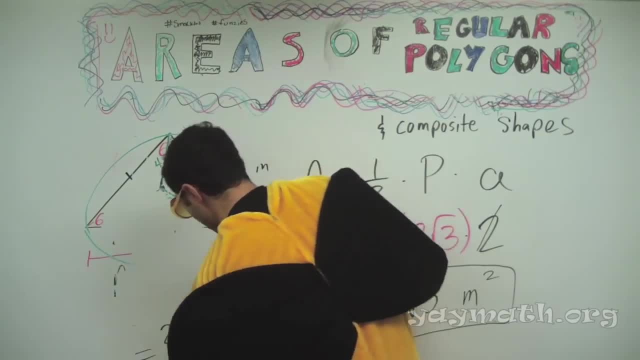 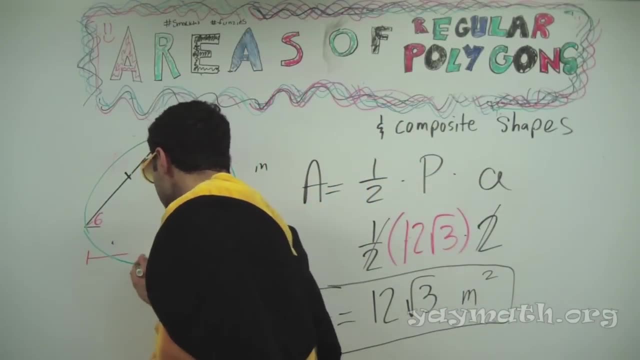 OK, A little, A little. A little is fine. Can I be dry? Is that OK, Please do It's not OK. Yeah, You have to erase what you do. Sure OK, These shapes can be really fun, or they can be really tricky. 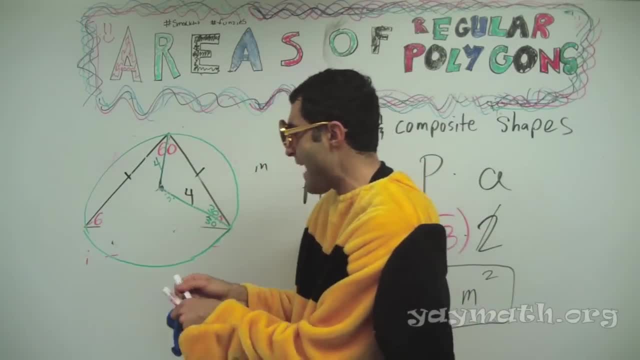 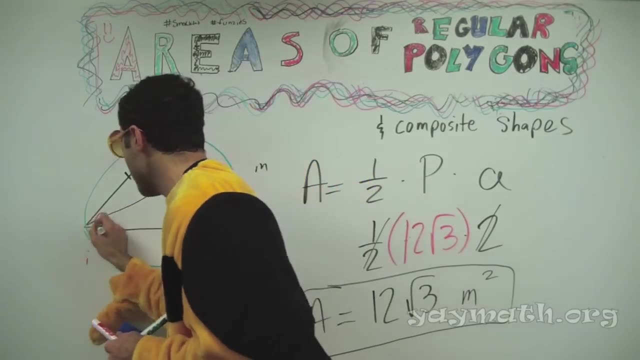 What we want to do is we want the area of the outside shaded region, That is, a great triangle, OK, The outside shaded region, And we have here, we have a path and we'll leave it as two, OK, Fifty-nine degrees. 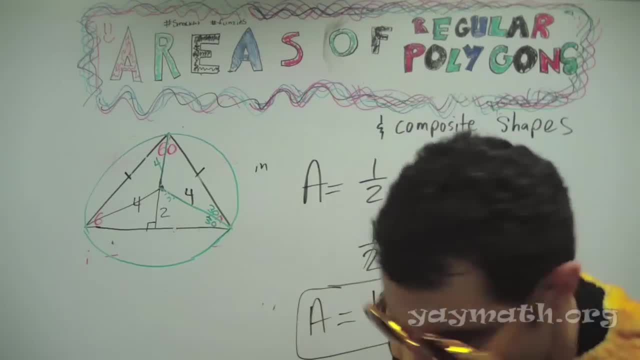 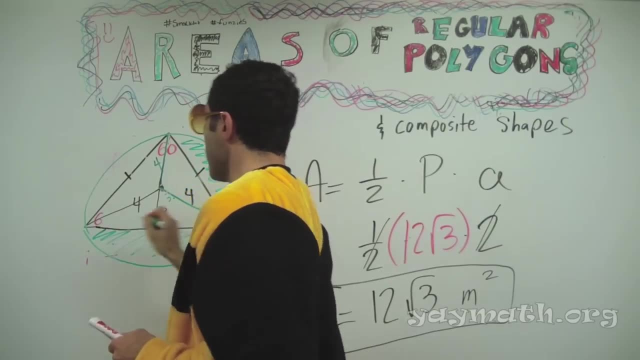 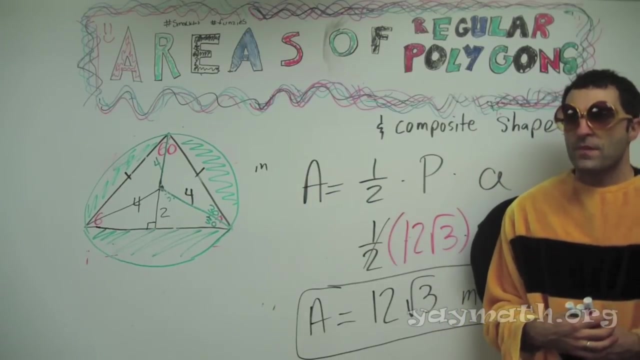 I'll shade that in green. I'll shade it in blue. Now, the challenging thing to understand about the shaded region is understanding the logic behind it. The logic behind it. Right, Let's get real. Let's get this off of you. 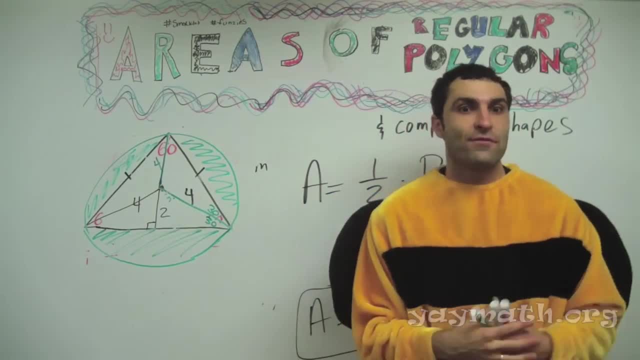 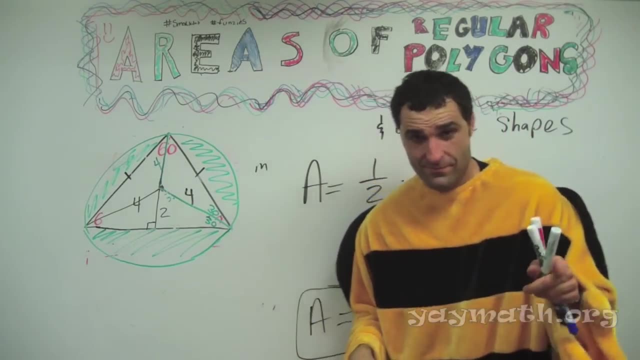 The logic behind the shaded region. Whoa Light flooding my eyes And you have like that little like you know, like Ridge Indents, Yeah, Yeah, And the nose pieces It's called commitment Point to this guy. 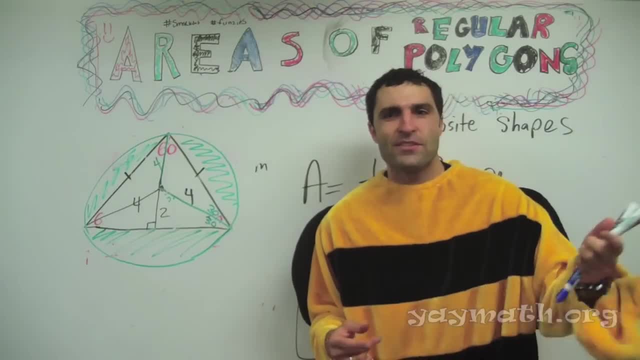 I think it's because you're reliable. That's why I point to you. Thank you, You're welcome. Thank you for taking it as a compliment. That's what I intended. So here we go. This is the entire shaded. The shaded region is what we want. 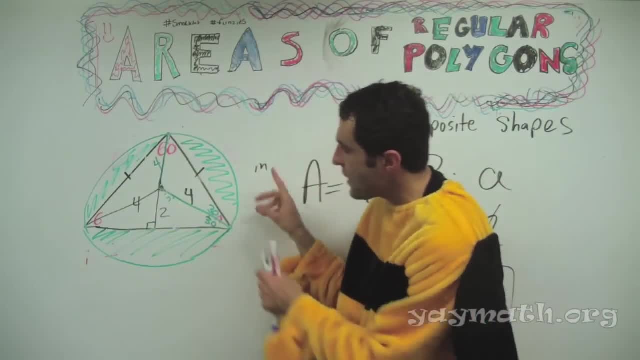 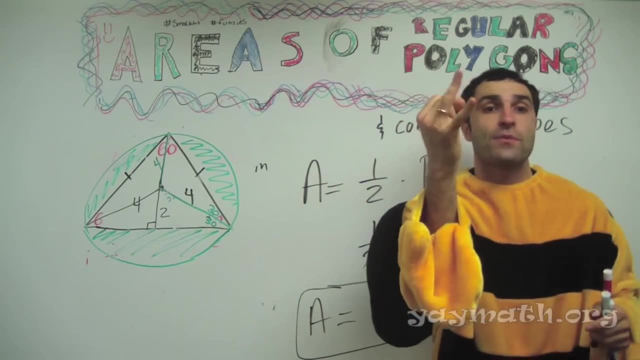 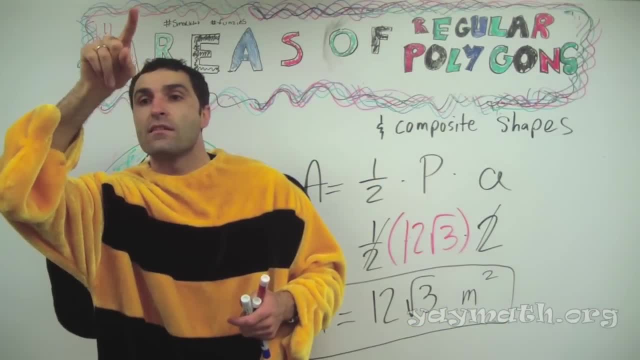 What's one area that we need? I know what to do We need. We need to know the area of one triangle, Of one of the mini triangles inside the triangle. Don't we know the area of the entire triangle? Isn't that enough? 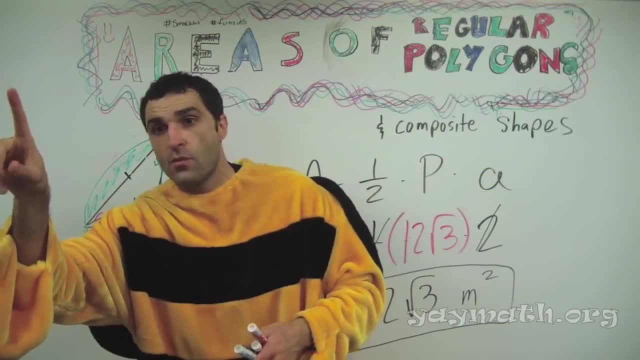 Ah, So we have the area of the entire triangle Just about there. What else do we need? Go ahead, Tell us We need to find the area of the circle And then we need to track the two areas so we can find the area of the outside part. 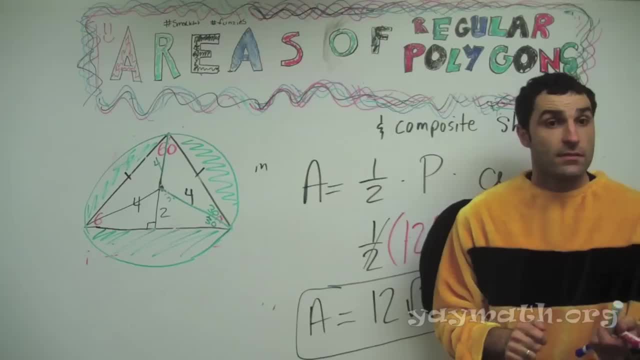 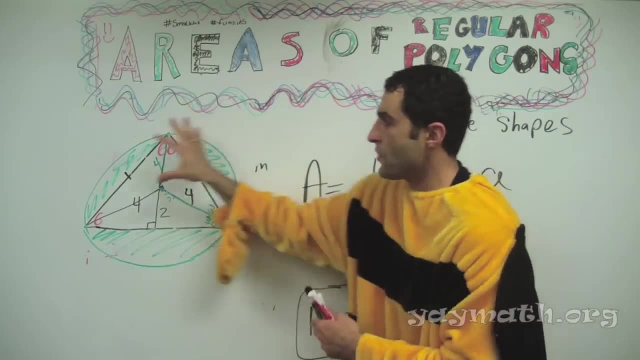 Be right along. It's basically like the walk around the pool, Like we have basically like a pool, Yeah, And then we have the deck And how much it's like around. That's right. If you have a triangular pool, circular deck, how much deck space is there? 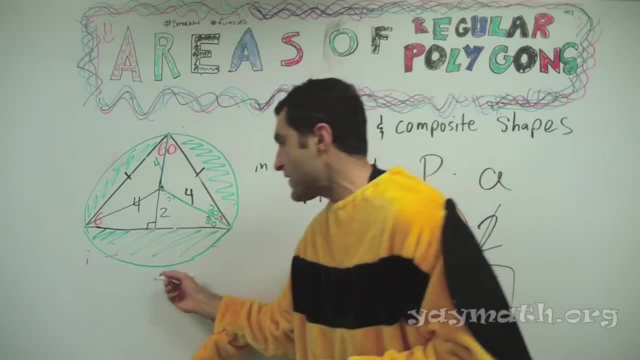 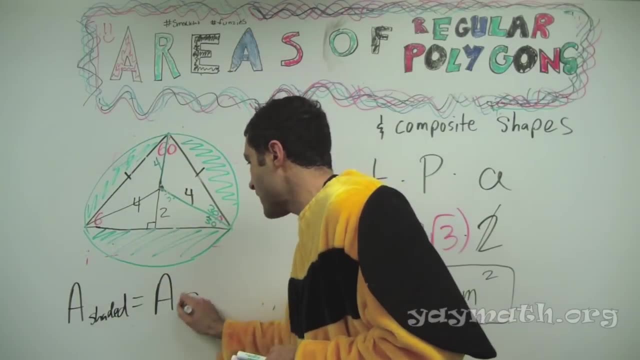 And that's the exact philosophy. The philosophy is this, and please write this down: Very important: Area of shaded equals area of the circle. So who's tuning in to what he said? First you get the area of the circle. Someone else say it? 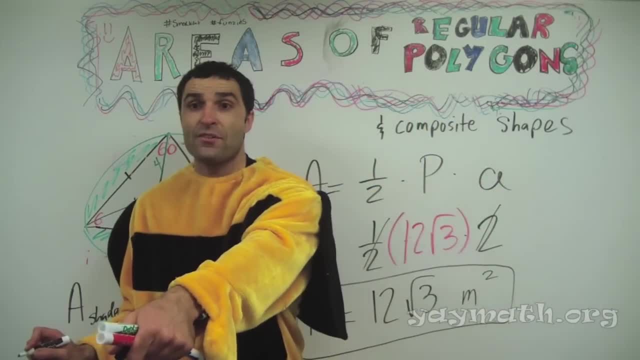 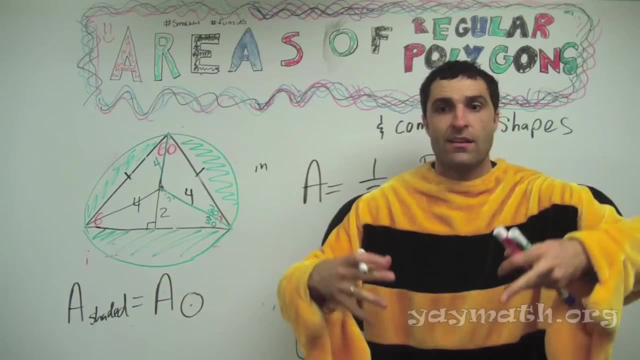 What do you do from the area of the circle? Someone else besides you two- because I'm glad you're really tuned in- You do area of the circle. Then you take what out of it? You take the triangle, Yes, The area of the triangle. 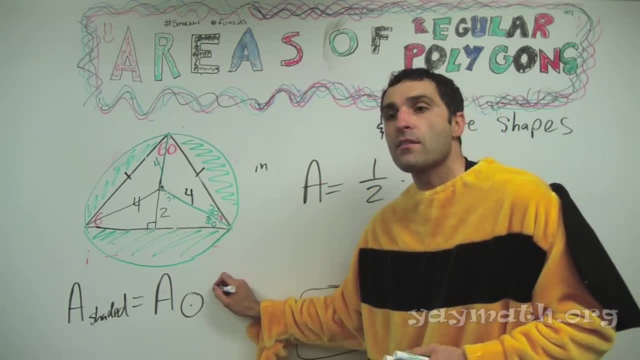 So what math am I doing? Minus, Minus Area of Triangle: Very good. Area of the triangle, Area of the shaded region equals the area of the circle minus the area of the triangle. Are we okay with that? Any questions? 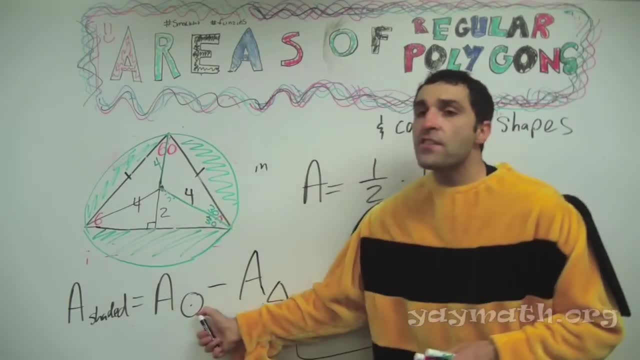 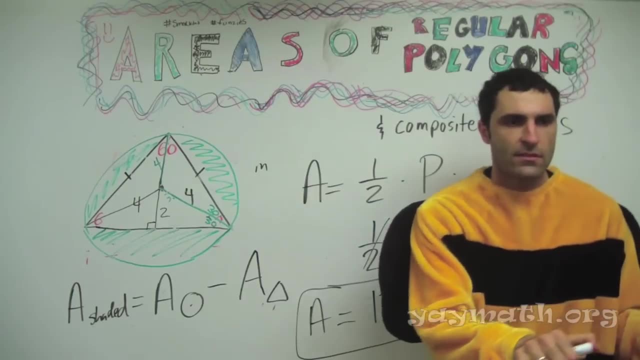 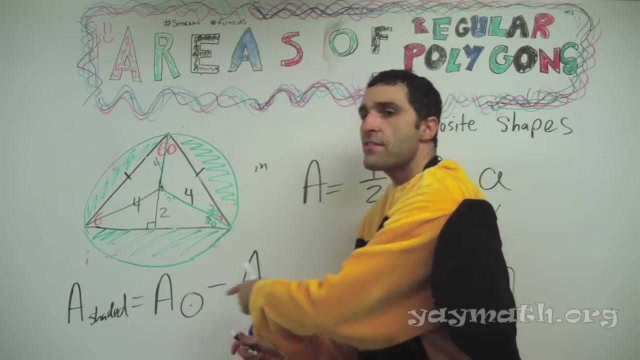 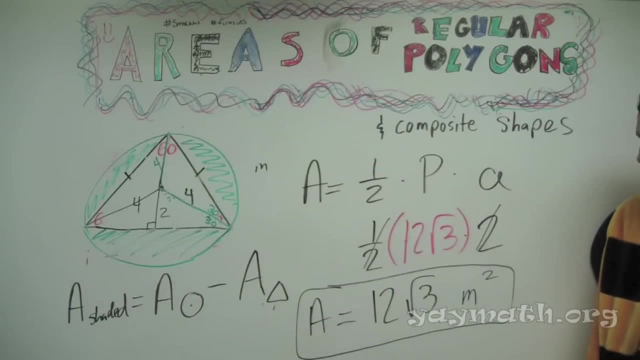 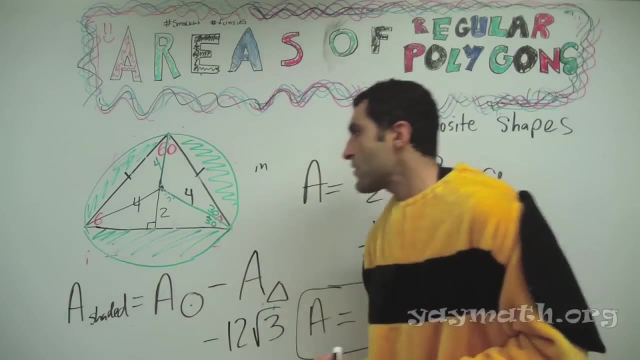 What can I fill in? You could fill in the area of the triangle- We know that We did that already- Which is 12 root 3 meters squared, So let's put 12 root 3 in here. Now we need the area of the circle. 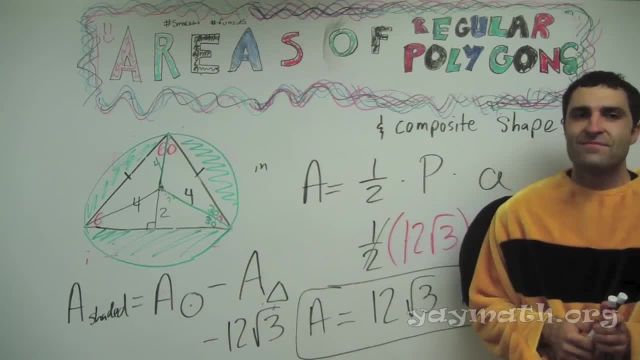 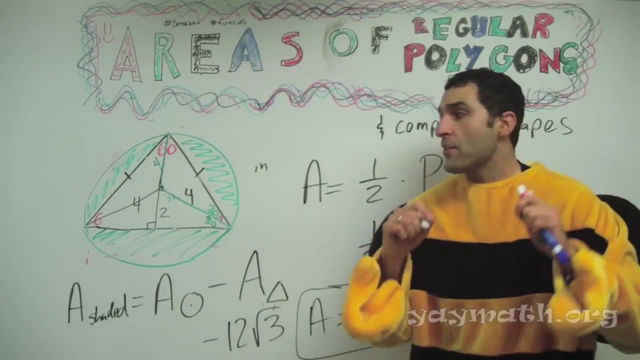 What we could do is: Do we have a measurement on the circle? Any measurement 360.. What is the formula for the area of the circle? It is A equals high R squared. High R squared. Put it down: Pi r squared. I wish I knew radius. 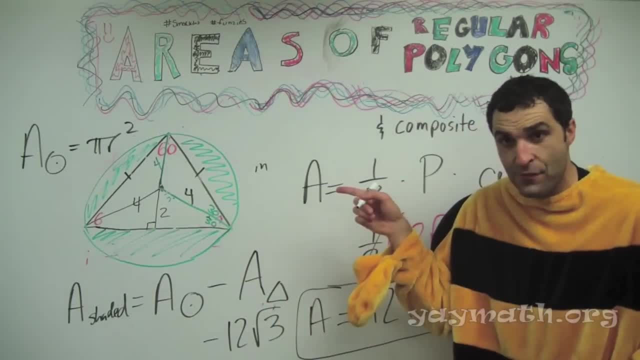 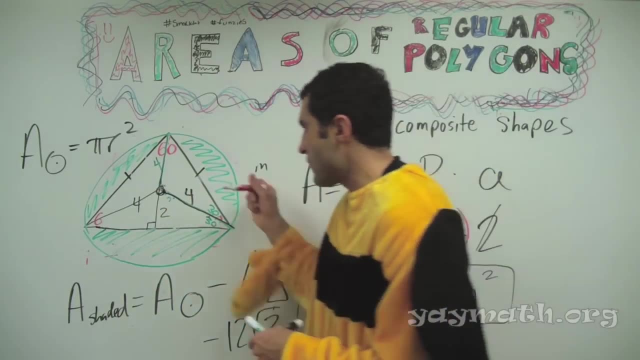 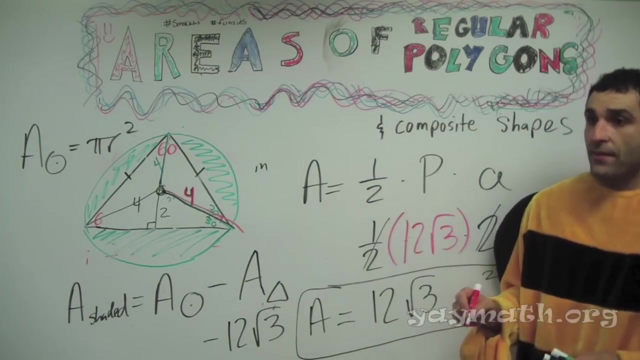 We do, we do. It's looking right at us. It's four. There it is. Oh, there we go. Four, that's outlining in red Radius, looking right at us. Four, What is the area of the circle then? 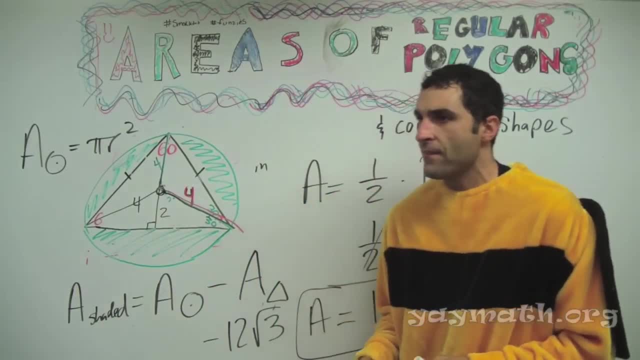 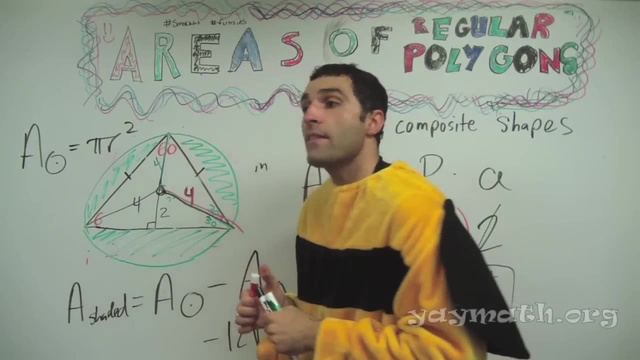 Tell us If the radius is four. try, try, Mr B man. If the radius is four and the area is pi? r squared, what would it be? Sixteen pi. Thank you for thinking it through. It's a lost art, isn't it? The act of sitting and thinking. 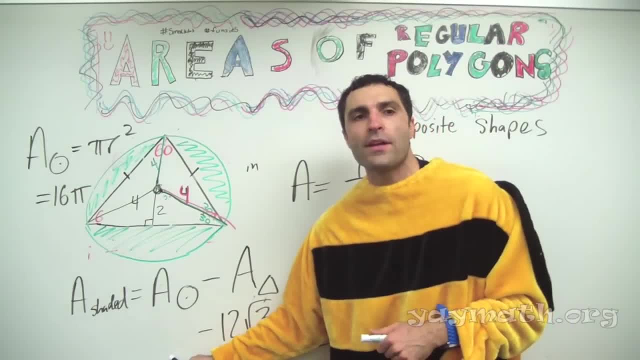 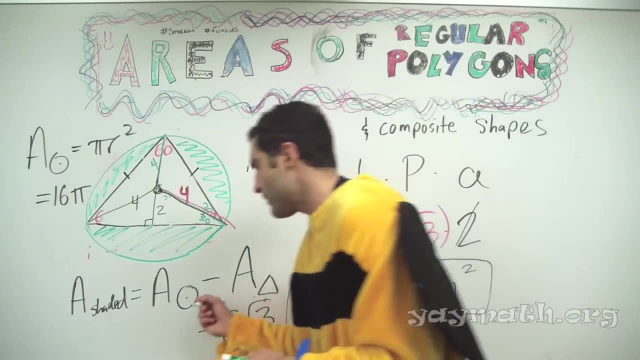 Let's put down the area of the circle before we conclude this problem. What's the area of the circle here, please? Oh, it's sixteen pi, Sixteen pi. So now the question is: I want some pi. Do these combine No? 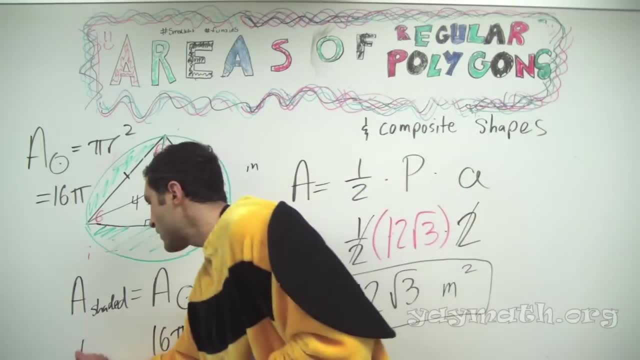 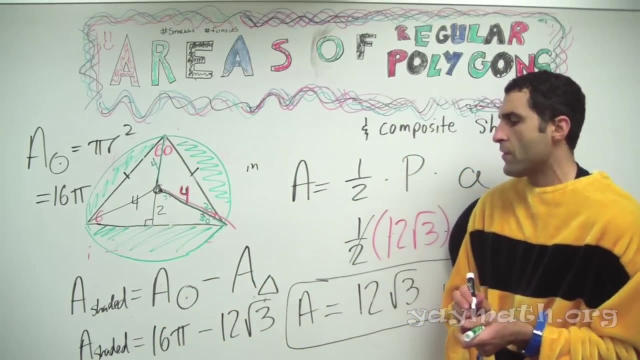 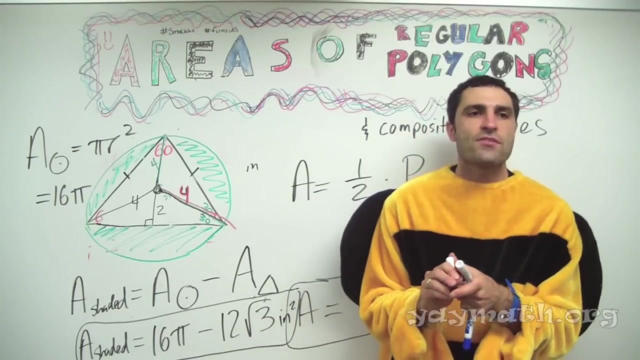 No, So we're done. And the shaded region is equals sixteen pi minus twelve, root three inches squared. Okay, now back to the story of Mr Smith, and then we're done. Mr Smith, my seventh grade teacher, at the end of one PE class. 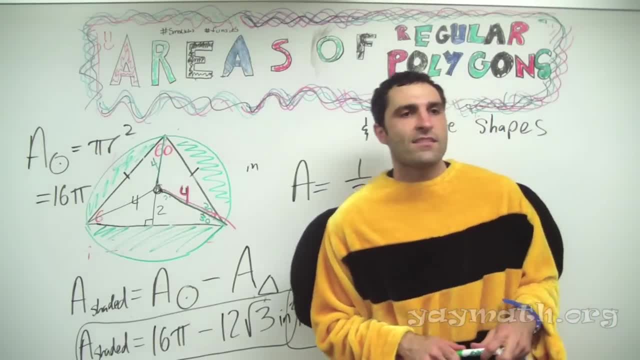 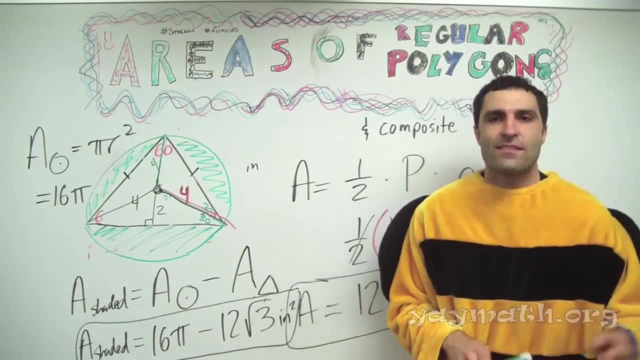 he said: tomorrow we're going to discuss the funky Kornhauser rule, What I'm serious. And then he said, okay, class dismissed. And then we would leave, And then the next day we would come to class. And then he would ask: 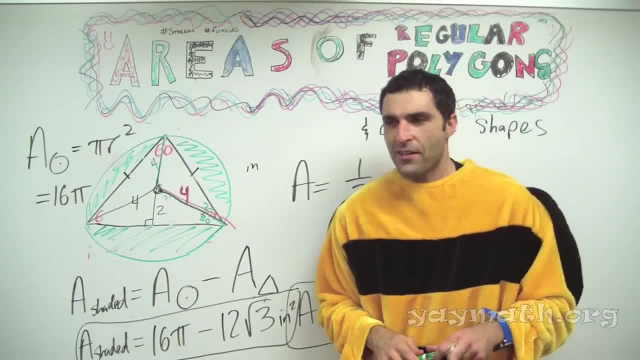 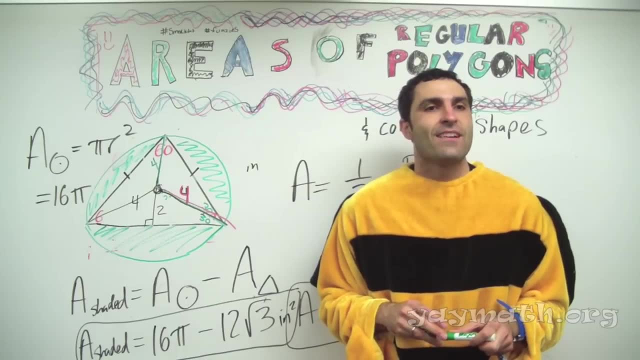 He'd be like Ecclesiastes or Cornelius or Smackdad- Disgrace. He'd say: what are we going to do today? And then the guy was like, oh, I don't know. He says, okay, just think about it. 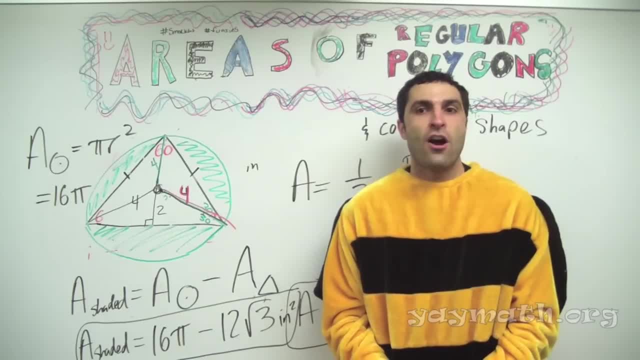 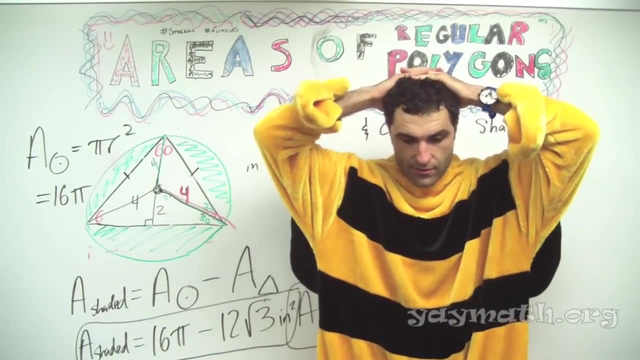 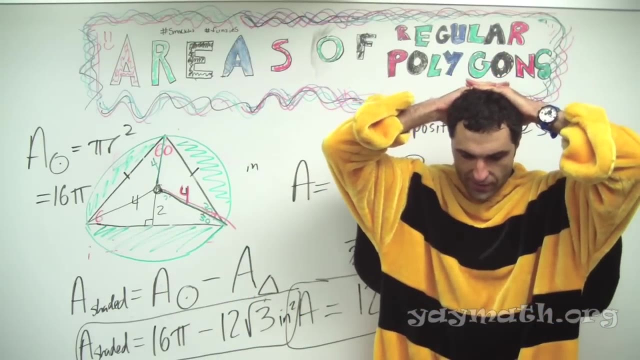 And we sat. We stood for like five long minutes And I'll never forget the look on his face. He was like this: Why did he forget too? He was thinking, He was thinking And he went like this: After five minutes he said: oh, we're going to go over the rule. 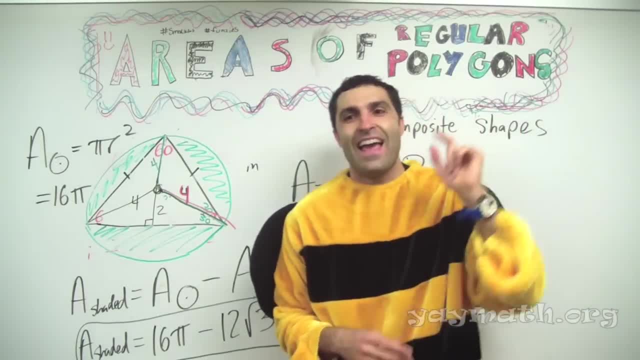 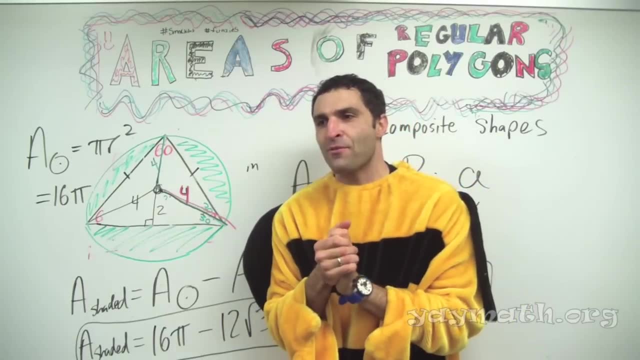 And he was like nice And I always thought that since then the act of long-term unbroken thought has been a lost art form. It was a beautiful moment. For five minutes we just let this dude just think And he just. 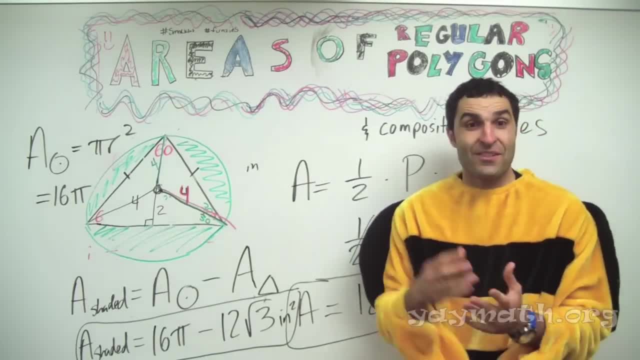 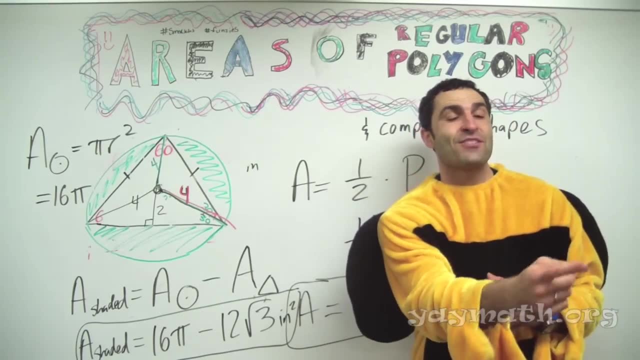 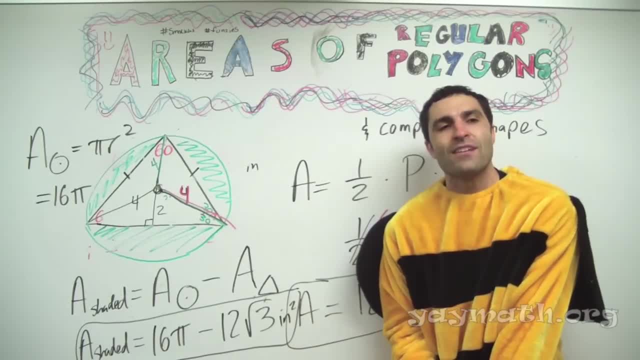 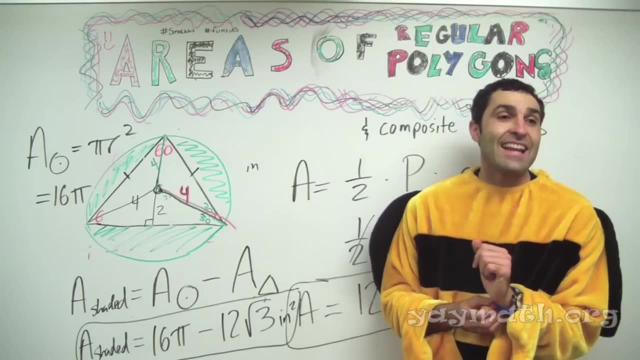 us to remember what happened the day before. It was really cool. I need to remember what you said. I know Me neither, Funky Kornhauser. It happened to me the other day Back in Maryland. It happened to me the other day For Father's Day. we went to a restaurant. 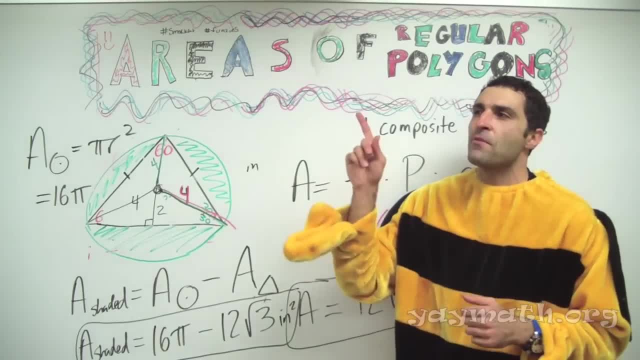 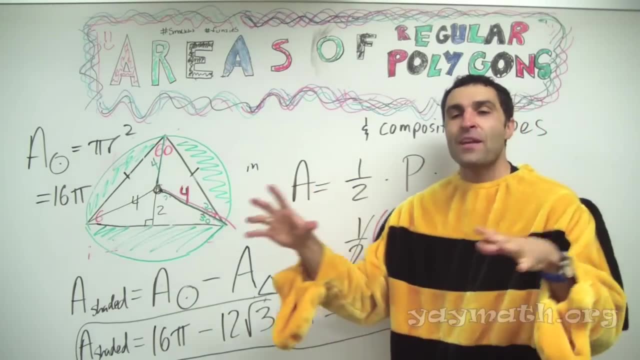 And I remember the waiter's name- It was Skyler- And I looked at him and I was like Skyler, Him, Yeah, Wow, Yeah, He had a beard. Really. He closed it And from then on we had a great experience, because I remembered